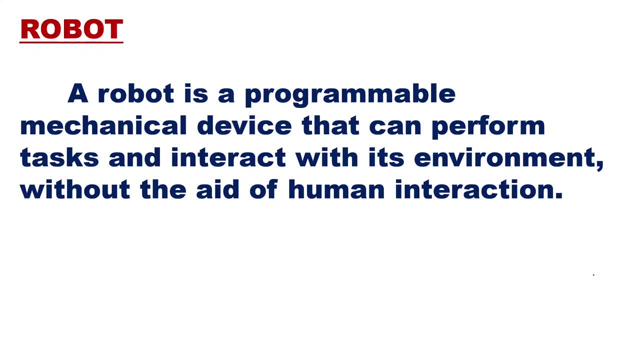 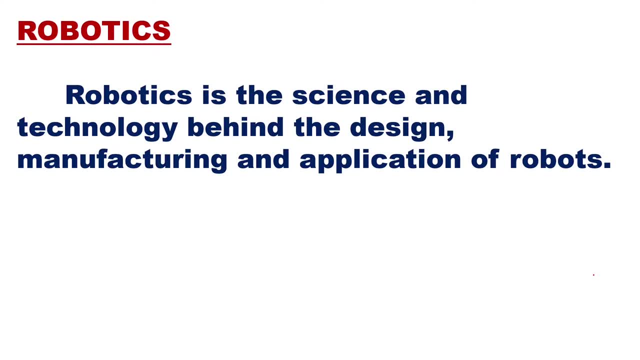 tasks and interact with its environment without the aid of human interaction. then what is robotics? robotics is a science and technology behind the design, manufacturing and application of robots. so, after knowing this field of robotics, and as the robot is the product of this field, we will go to 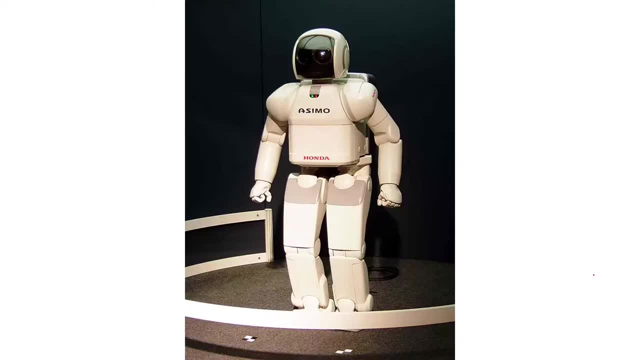 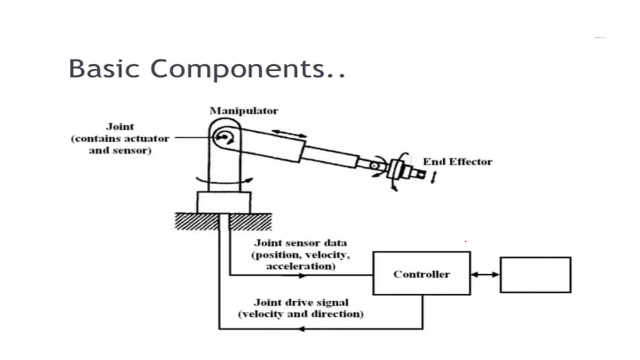 the basic components of a robotic system. so here you can see an image of a robot. now, here we will see the basic components of a robotic system. so here the first thing, what we have is the base. so here you can see, this forms the base. okay, this is the base part of the robotic. 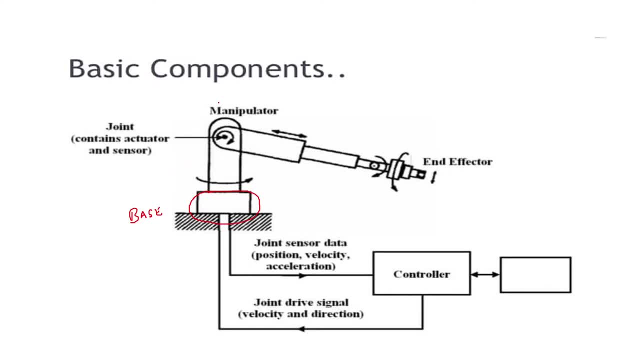 system. now, here you can see the most important manipulator. this is the manipulator arm. this is the transmitter. then here you can see joint. here is the joint. now the joint contains actuator and sensor. this is the arm. at the end of this arm you can see there is a end effector which is 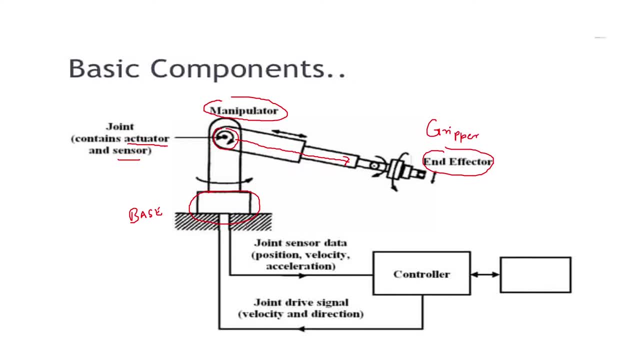 also called as gripper, which is also called as gripper. then there is a connection for the signals. so here you can see joint sensor data. so whatever sensors are there get connected to the cognitive system and we know the articulator, which is blade visual Lor. I don't know how it works, but 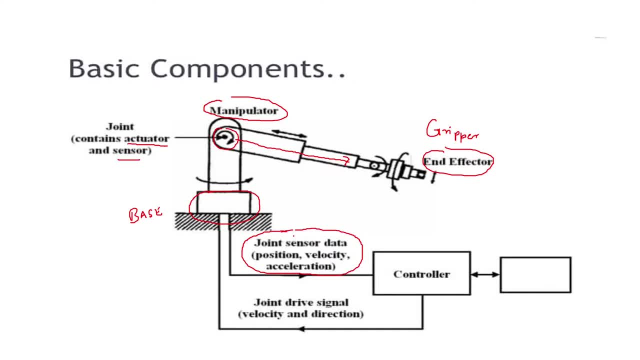 it looks like a medium, so we will see these things, create it and create a photograph and also inject the arm into our bodies at the joint. that data now. in that data you can have your position, velocity, acceleration. that will be given to the controller here. this is the controller. 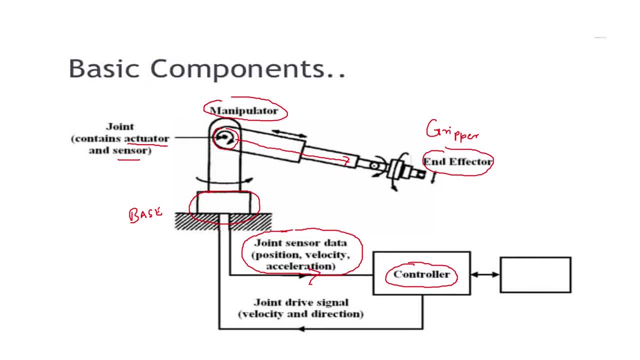 which is going to take the inputs, process the inputs and, depending upon its program, it is going to give the output to the actuator to act on. then, once it is executing the controller has executed everything, it will give out a signal- this is called a joint drive signal- and which will decide the 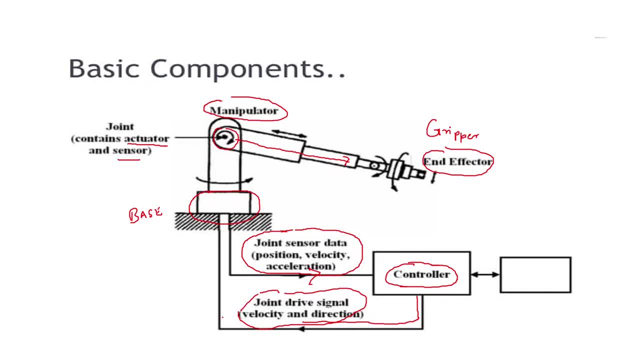 velocity and direction which the actuator has to perform. that will be given back to the system, which is your robotic system, and then this particular actuators will work and, based on that, this joint will work and based on that, this arm will work and based on that, this end effector will give you the 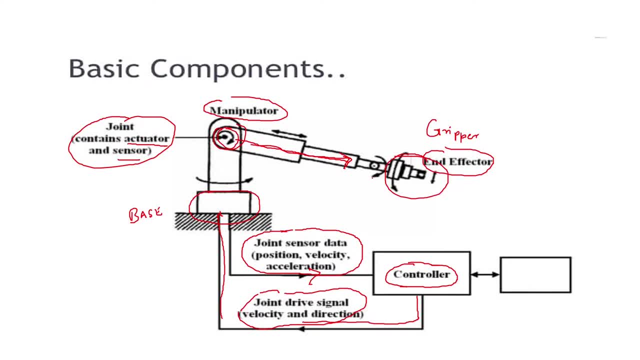 output should be distributed. then that is the last task. whether you have to pick something or whether to pull something, whatever it is that gripping work can be done. the end now. here you can see a controller and for this the power source is given here. this will be your power source, which will be given to the 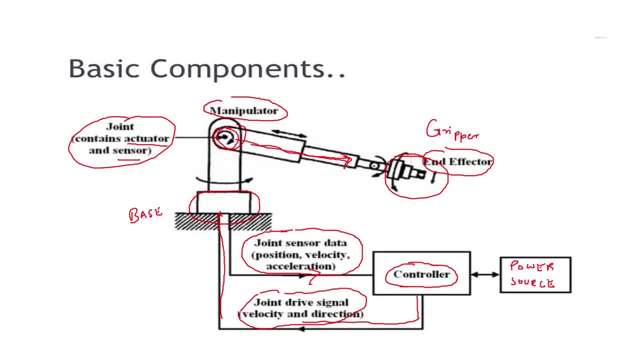 controller, okay, and because of that, because of this power, the controller will be working and hence your working okay. so here the main important points. what we see is your manipulator, the one joint over here, which is going to manipulate all your actions, okay, and then you have an end effector, then you have what are actuators? okay, and then 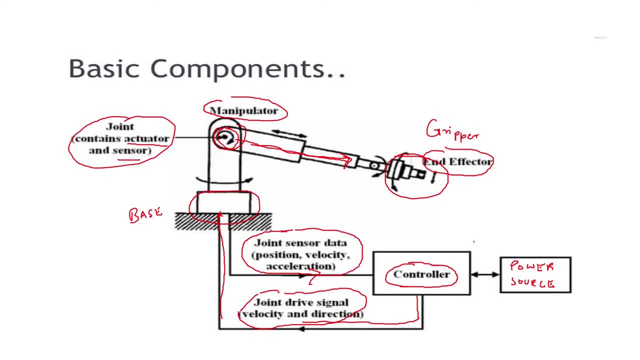 the elements which join this actuator and the joints are called as transmissions. okay, and then you have a controller which provides the intelligence that is necessary to control the manipulator system. then you have sensors which will sense and give the input signal to the controller. okay, so these are the basic. 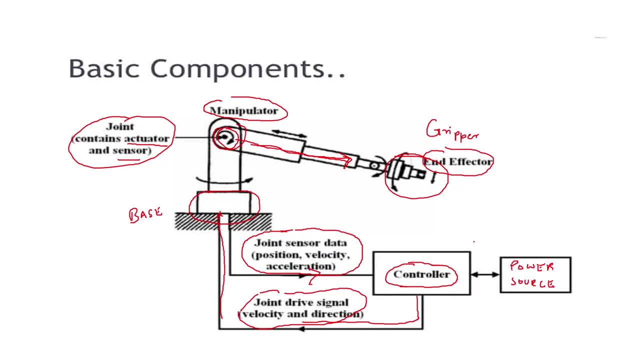 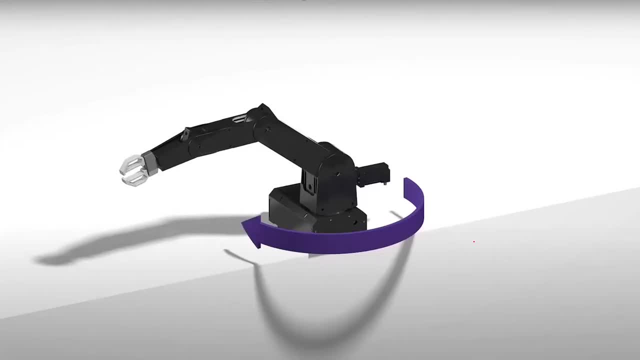 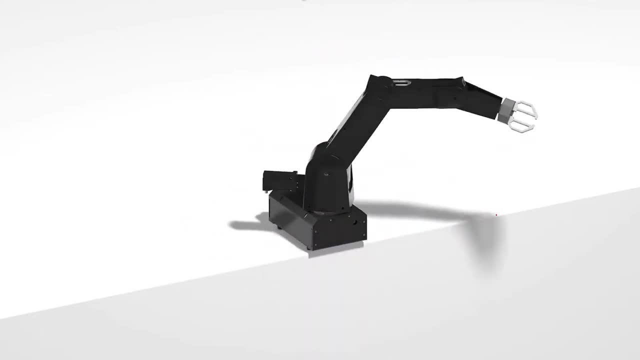 components of a robot system. yeah, so then we will see how does it function. so here you can see how it is functioning. so here you can see the robot arm, the gripper. so here you can see the gripper and the robot arm how it is moving. so in this way you can show the movement of 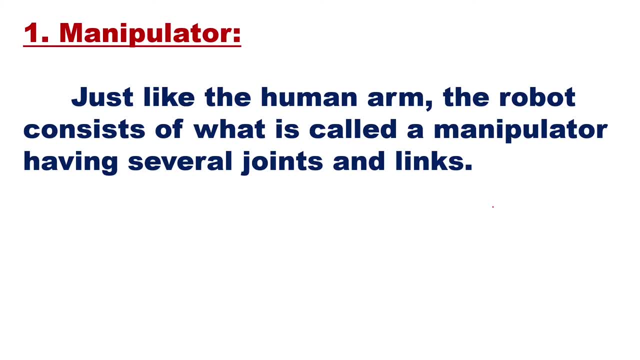 the robot. then we will come to see what do you mean by the manipulator. now, just like the human arm, the robot consists of what is called as manipulator, which has several joints and links, so it is a very important part of your robotic system, that is, manipulator arm. so here the most important mechanical 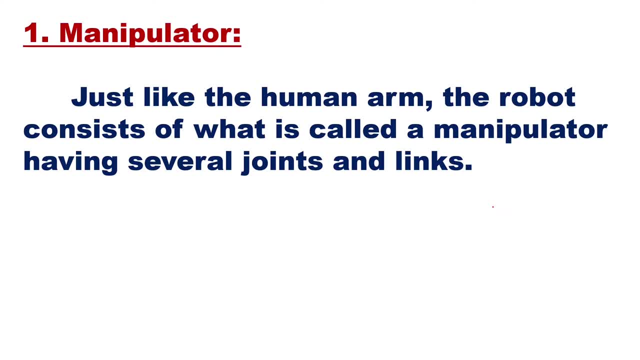 configuration of the robot is the manipulator arm. now, this manipulator arm consists of several separate links making a chain. this arm is located relative to the ground, on either a fixed base, as we have seen in the first diagram, or a movable base. it has a free end, the free end which we showed near the end. 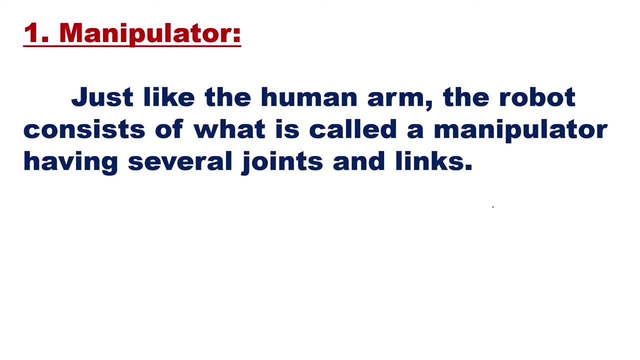 effector. it has a free end where an end effector or gripper, or sometimes a specialized tool holder to hold or any power device, say like a drill, is attached to it. okay, so this is basically an arm which manipulates the functions which will do the required tasks, and it consists of several joints and links. 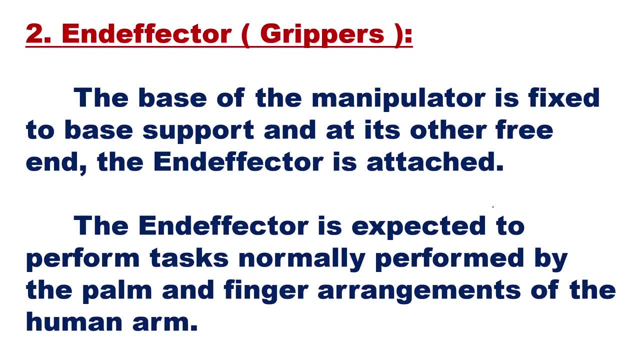 then we'll go to see. what do we mean by end effector? the last part of the part where the gripping of things used to take place. so here, according to the definition of it, it is the base of manipulator which is fixed to the base part, base support, and at its other, free end, the end effector is attached, the end. 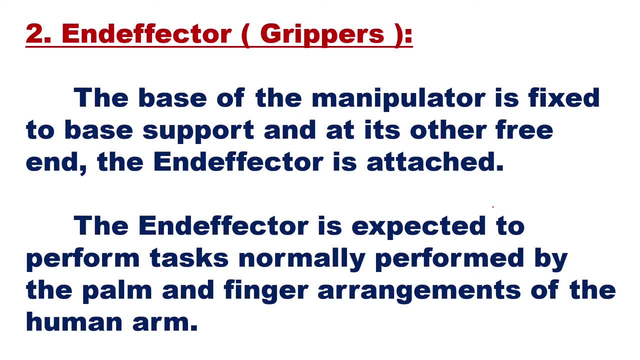 effector is expected to perform tasks normally performed by the palm and finger arrangements of a human arm. so if you resemble this with a human being, then the human arm, that is, the palm and finger of the hand, that will be your end effector. that will be the gripper. the fingers are used to grip and hold certain. 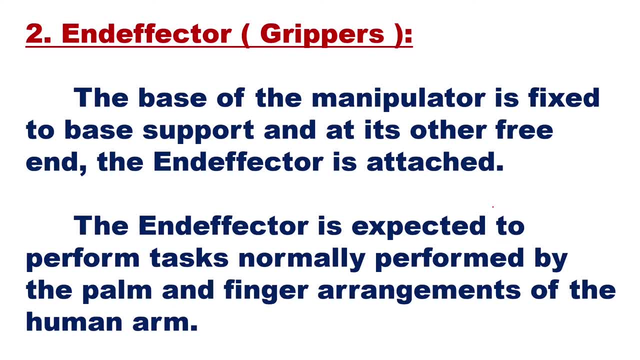 things, okay. so that is where your end effector of a robotic system will come into picture. so it is the a gripper or end of arm, okay, which is mounted on the wrist of the robot manipulator arm. so there is a wrist of a robot manipulator arm, it is mounted on that, this end effector is mounted on. 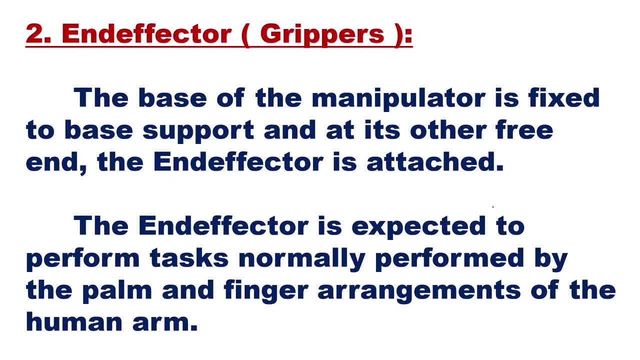 that a robot does a variety of tasks for which various tooling and special grippers are required to be designed. okay, a manipulator. the robot is flexible and adaptable, whereas its end effector is task specific. so its end effector will be exactly doing what task is given to it. it will either 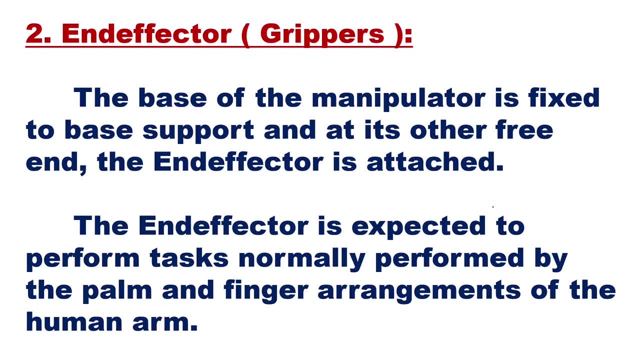 hold or grip. in that way it is going to do a specific task, so it is called as end effector. that is the effect at the end which is going to grip certain things, which is going to give a grip and hold certain things. then we will go to what. 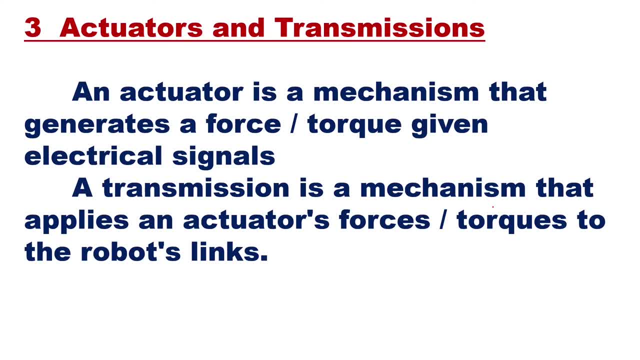 are actuators and transmissions, then here, actuator is a mechanism that generates a force or torque. force or torque a given electrical signals, or a transmission is a mechanism that applies an actuator forces and torques to the robot links. so here, what is actuator? now, actuator is a mechanism for activating a certain process. 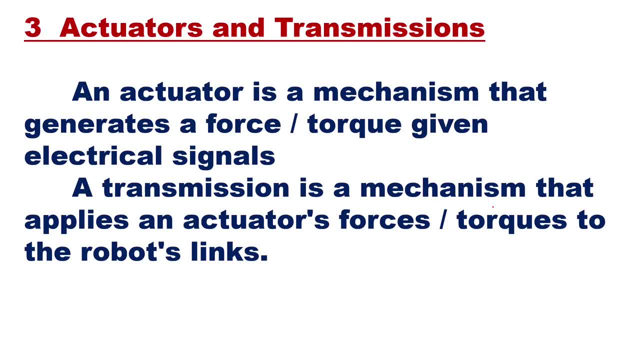 actuator is a mechanism for activating or doing certain process or control equipment by the use of. you can use pneumatic, hydraulic or electronic signals. you can use those signals which will be input and those signals will make the actuator to actuate things. it is going to activate the 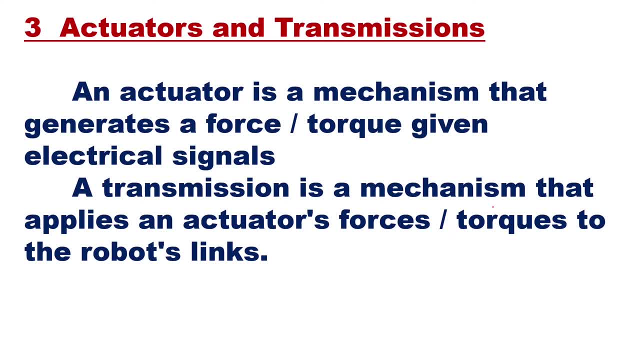 process and the process starts. so actuary is a mechanism for activating process. okay then, what is our transmissions now? these are the links, these are the elements between the actuator and the joints of the mechanical linkage. so the which comes in between, which joins the actuator and the joints of mechanical linkage, is your. 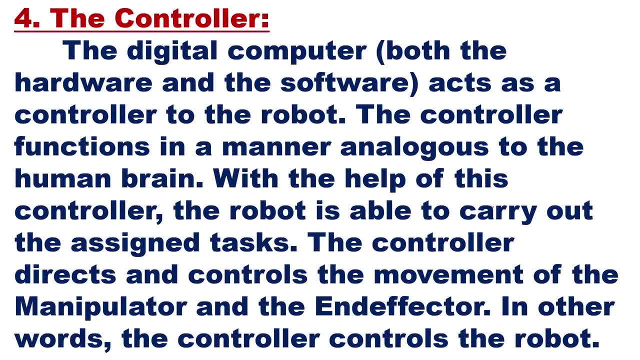 transmissions. then we'll go to see. what do we mean by the main part, that is, the controller. the digital computer, both the hardware and software, acts as a controller to the robot. the controller functions in a manner analogous to the human brain, so you can resemble this a controller to a human brain, because it is going to do the important work of decision making. 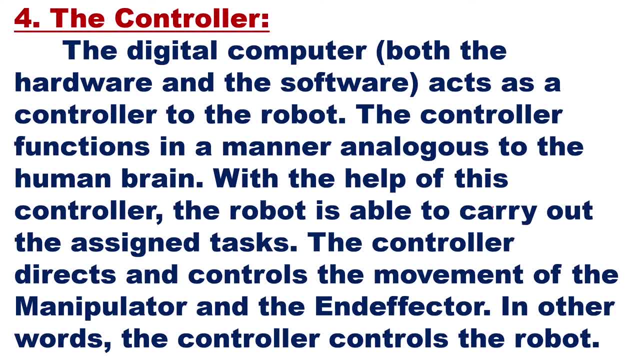 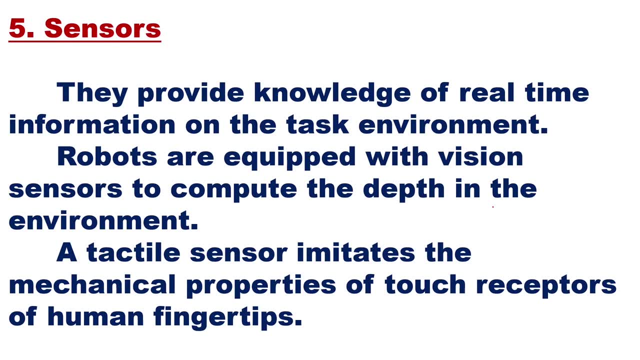 with the help of this controller, the robot is able to carry out the assigned tasks. the controller directs and controls the movement of the manipulator and the end effector. in other words, the controller controls the robot. then we'll go to see what are sensors. they provide knowledge of real-time information on the task environment. 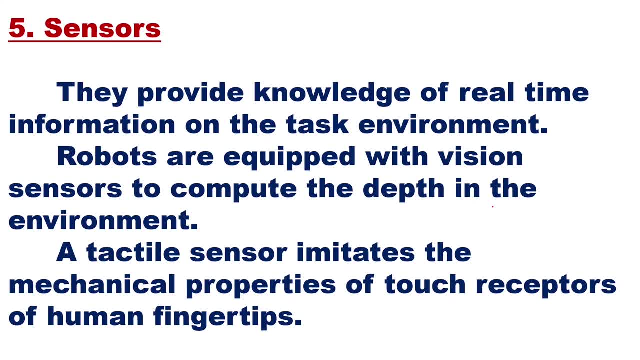 so you in the environment, whatever inputs you are going to take, that will be sensed by the sensors. robots are equipped with vision sensors to compute the depth in the environment. they are also equipped with a tactile sensors which imitates the mechanical properties of touch receptors of human